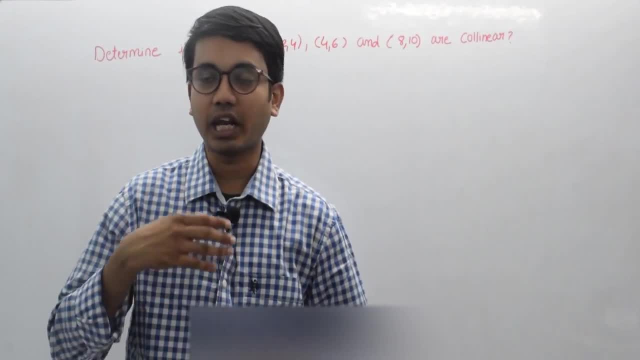 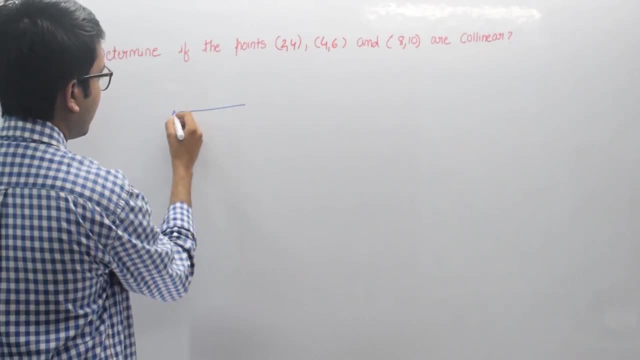 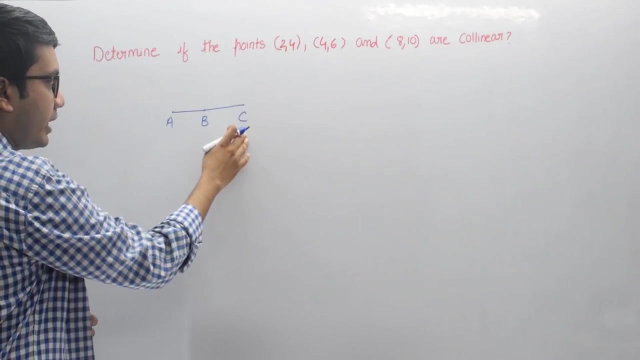 A set of points are said to be collinear if, and only if, they lie on the same straight line. For example, let us take three points: A, B, C. These three points are collinear if, and only if, they lie on the same straight line. You can see A B C lie on the same. 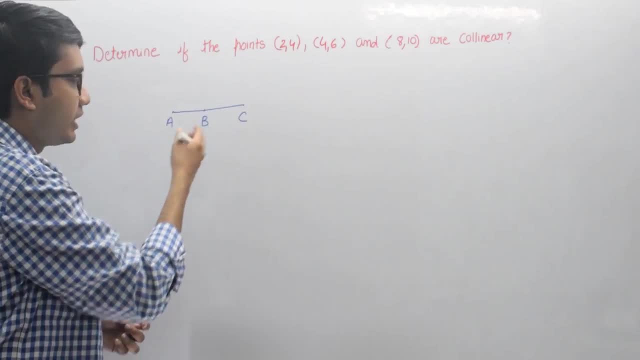 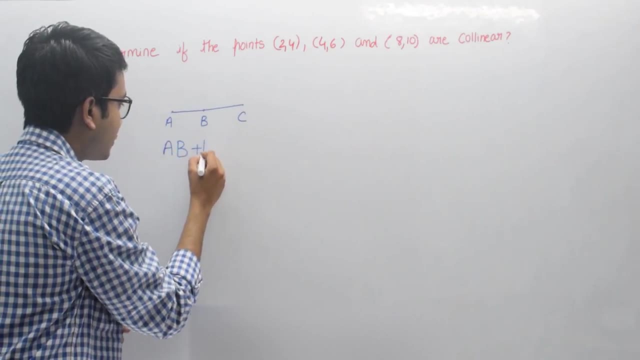 straight line. The important condition for collinearity is: if they lie on the same straight line, then A B plus B, So A B C lie on the same straight line. So A B C lie on the same straight line. 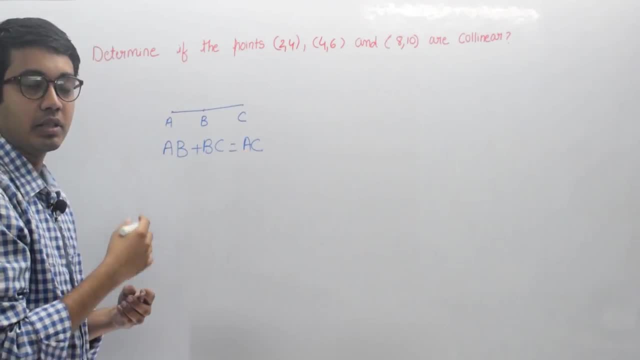 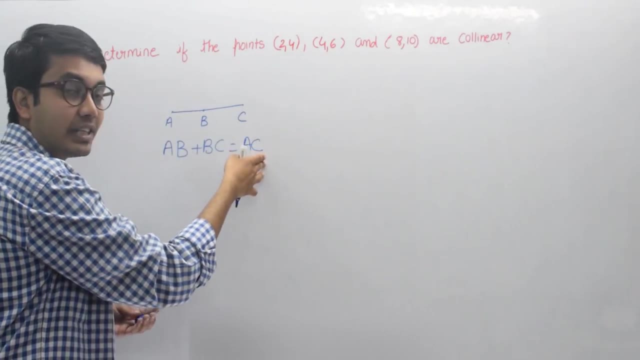 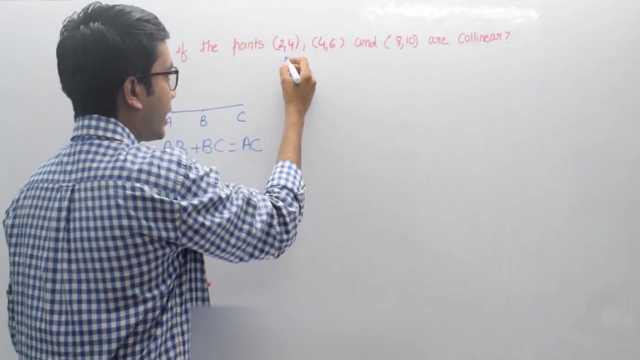 BC should be equal to AC. That is, the distance between the two points A and B, plus the distance between the two points B and C should be equal to the distance between the two points A and C. So we will apply the same concept here. Let us take this 2 comma 4 as A and this 4 comma 6 as B. 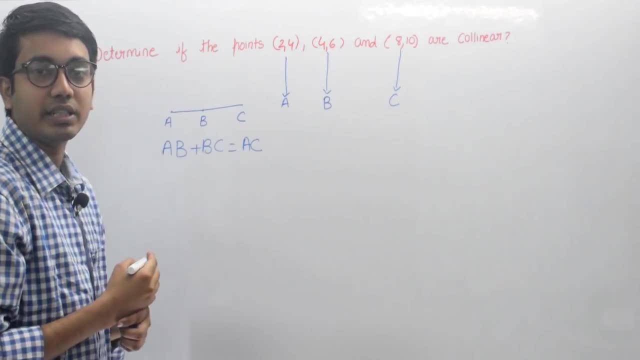 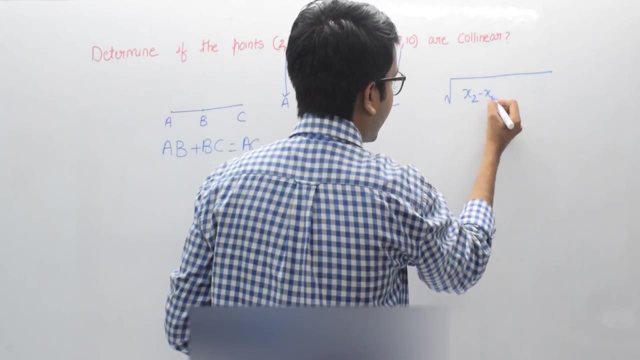 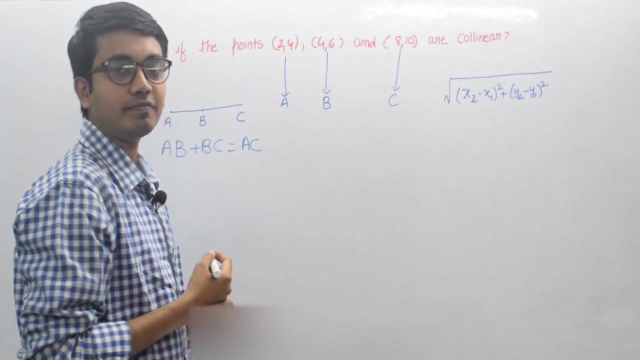 and 8 comma, 10 as C. What is the distance between two points formulae? The distance between two points formulae is square root of x2 minus x1, whole square, plus y2 minus y1, whole square. So first let us find out the distance AB. 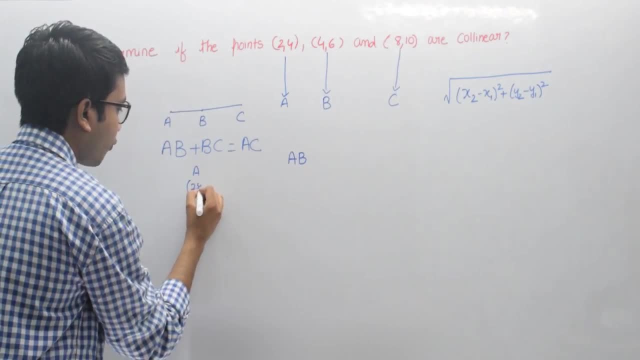 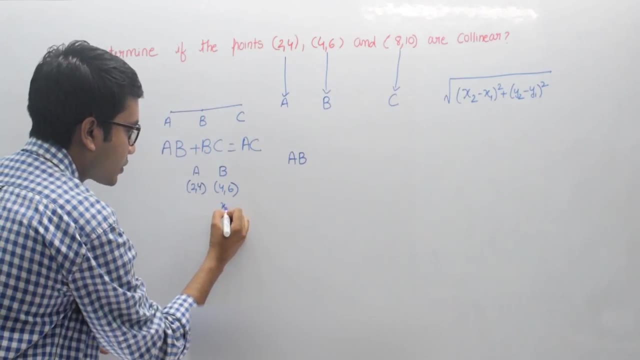 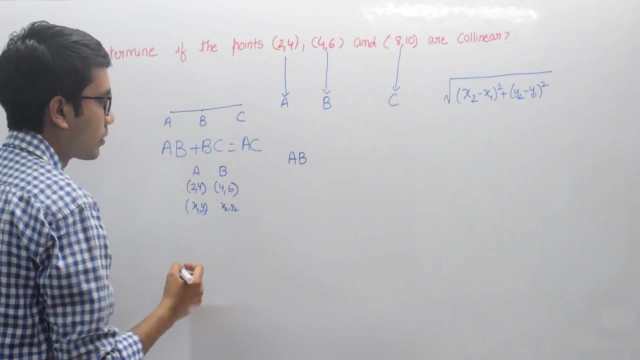 We know that the point A is 2 comma 4 and point B is 4 comma 6.. Let us take this point as x2 comma y2, I mean B. Let us take the point A as x1 comma y1.. So we will apply this formulae. 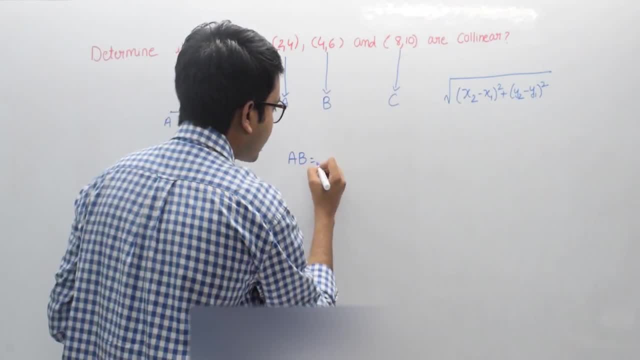 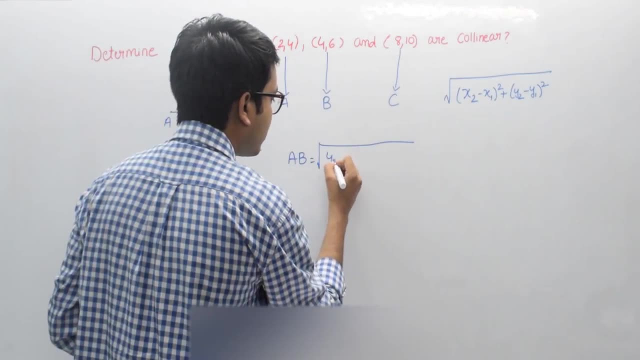 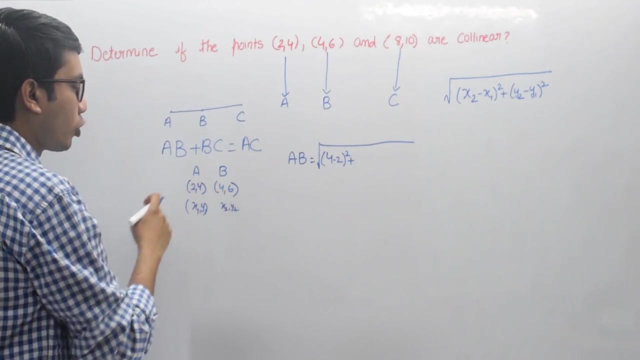 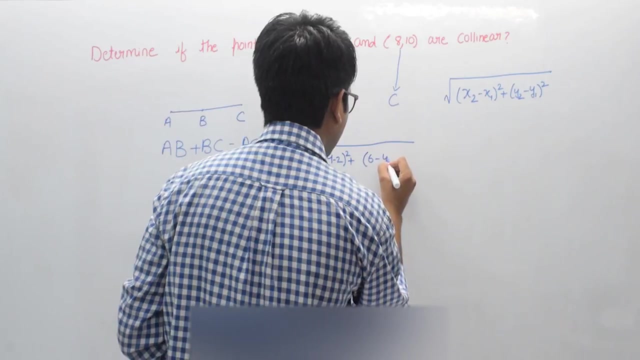 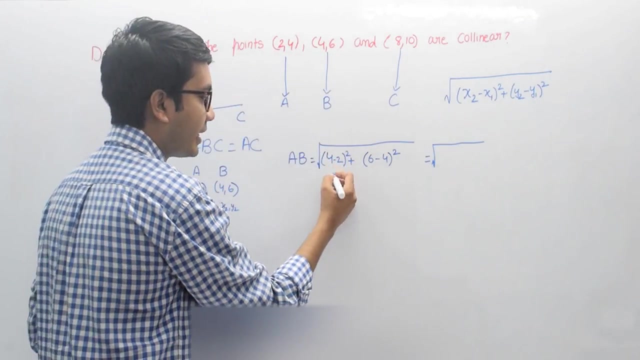 here to calculate the distance between A and B. So this will be equal to square root of x2 minus x1 whole square. 4 minus 2 whole square, plus 6 minus 4 whole square. What I did: y2 minus y1 whole square. So this will be equal to square root of 4 minus 2 whole square is: 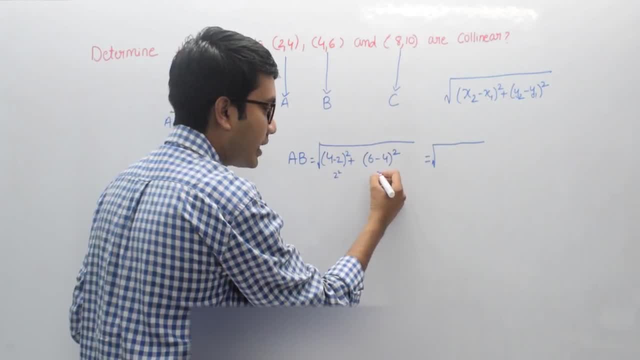 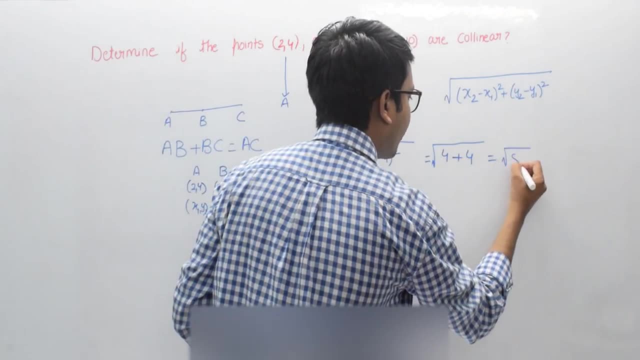 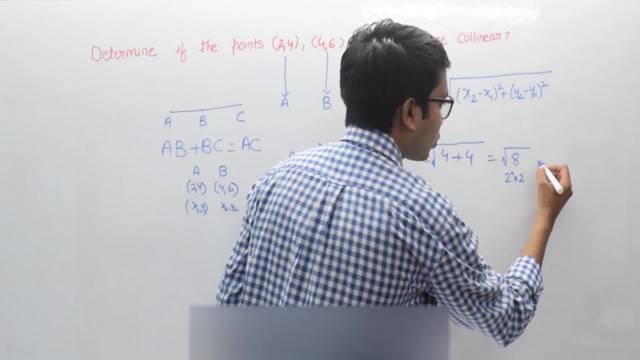 2 square and 6 minus 4 whole square is 2 square. So this will be 4 plus 4.. This will be equal to square root of 8.. So this 8 can be written as 2 square into 2.. So this will be equal to 2 square. 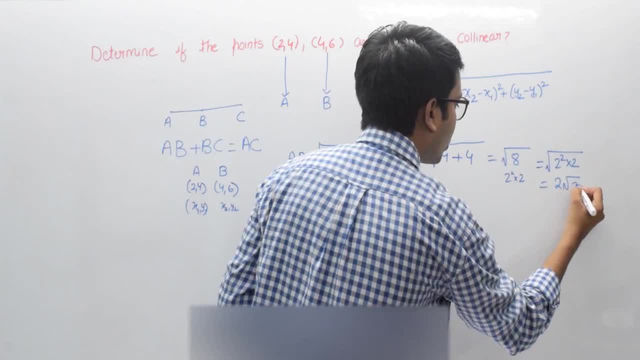 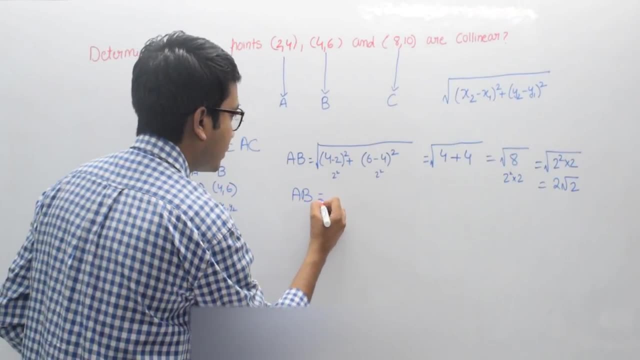 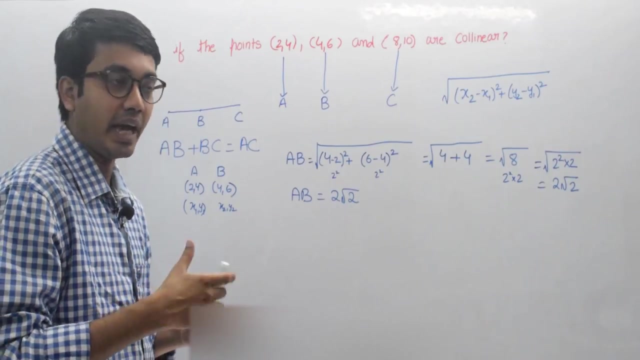 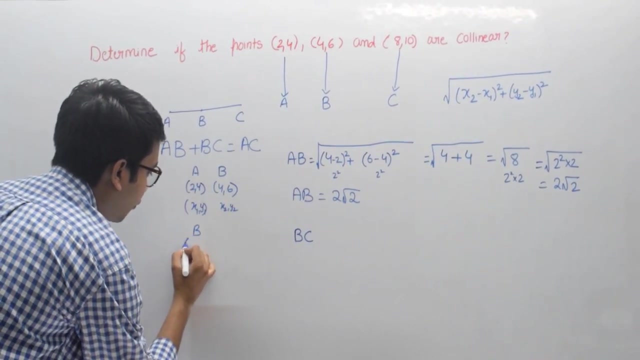 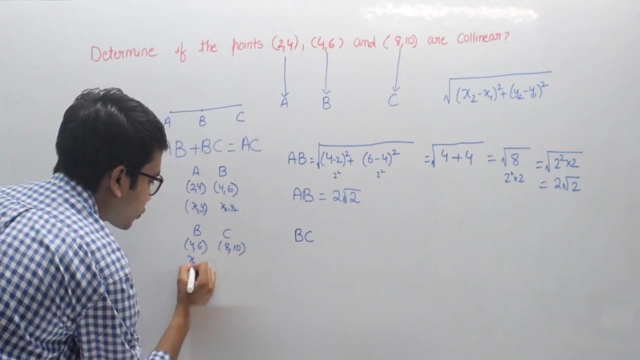 into 2, which is equal to 2 root 2.. So finally I got AB as 2 root 2.. Next we will find the distance between B and C. What are the points? B is 4 comma 6 and C is 8 comma 10.. So this I will take x1, y1,, 4 and 6 and. 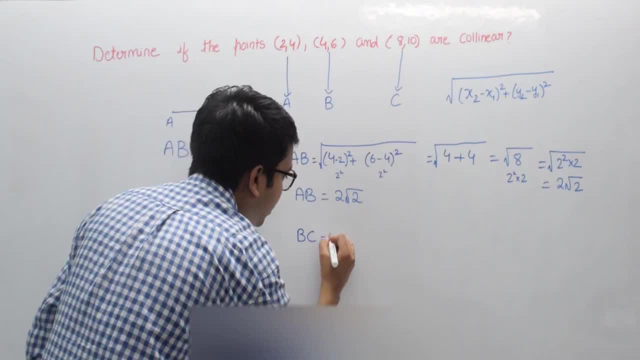 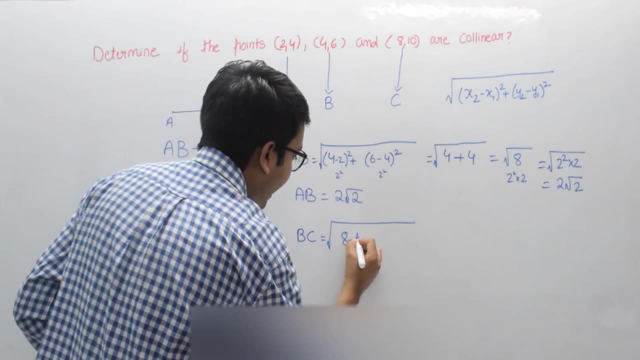 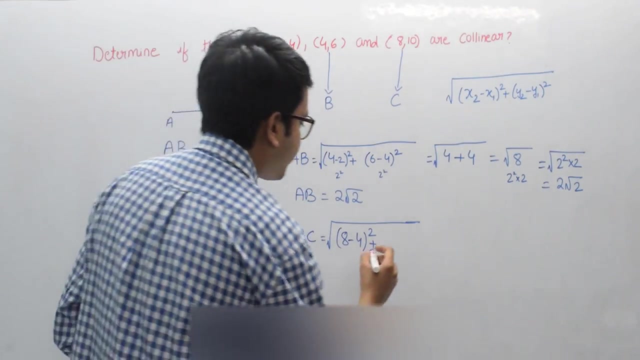 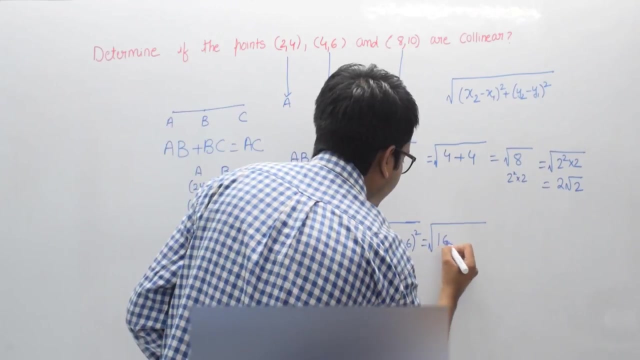 this 8 and 10, I will take x2- y2.. So I will apply the same formula here: square root of x2 minus x1, whole square, that is, 8 minus 4 whole square. plus 4 minus 4 whole square. 10 minus 6 whole square, So this will be equal to 16 plus 16.. How 8 minus 4 is 4 square, that is: 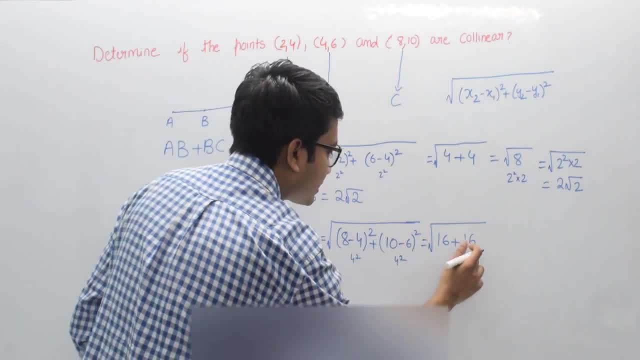 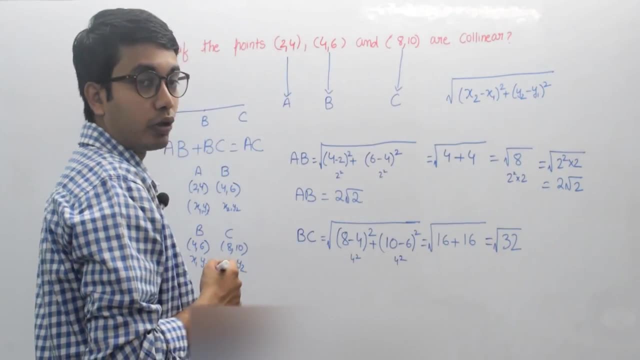 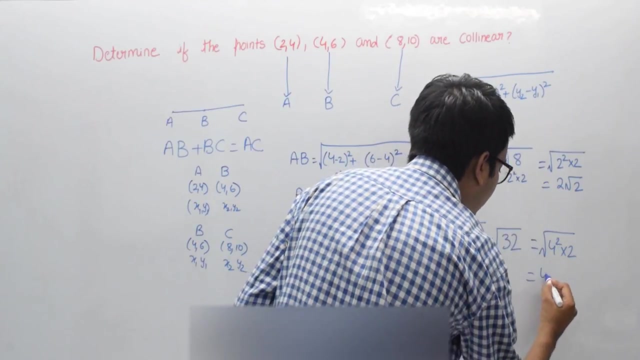 16.. 10 minus 6 is 4 square, that is 16.. So this will be 16 plus 16, which is equal to square root of 32.. Now this 32 can be written as 4 square into 2, which will be equal to 4 root 2.. So BC is: 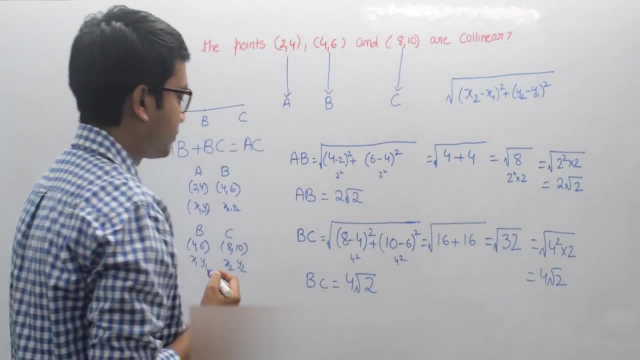 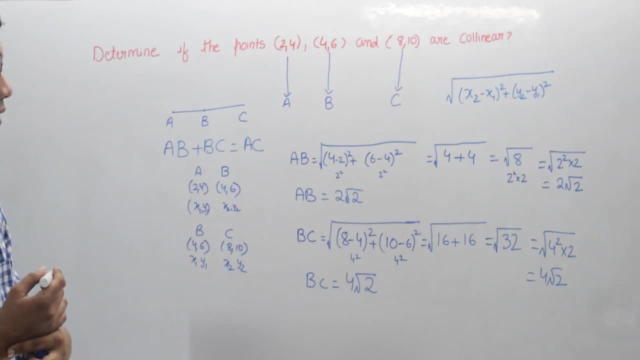 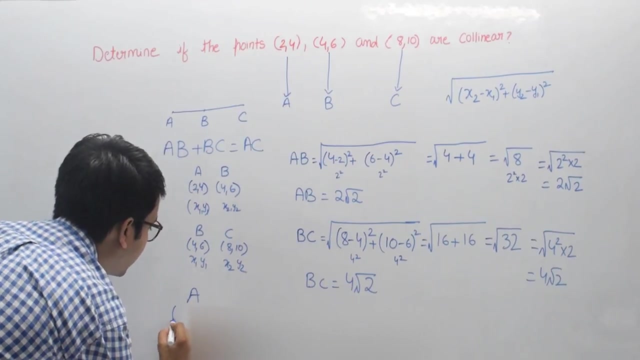 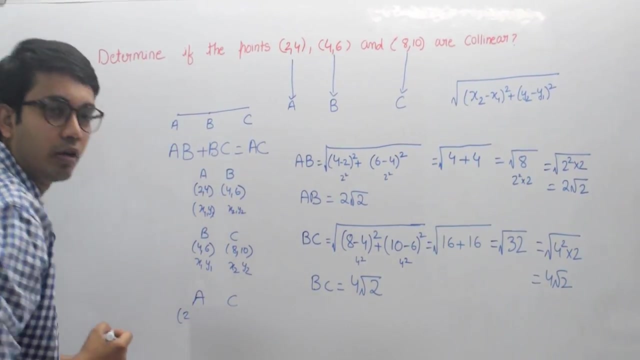 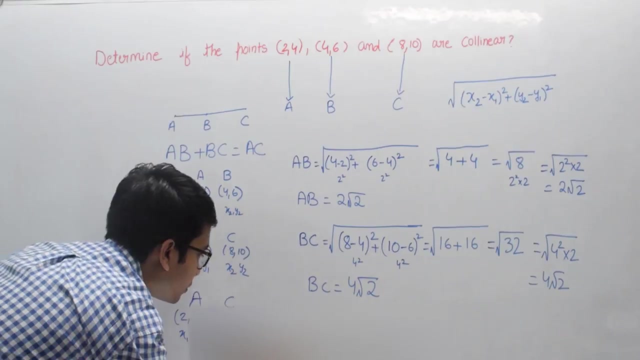 equal to 4 root 2.. Now I will try to find out CA or AC. So A is 2 comma 4 and C is 8 comma 10.. So this will be x1 y1 and this C will be x2 y2.. So AC will be. 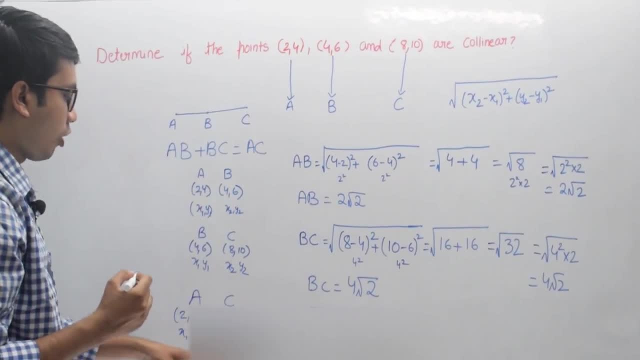 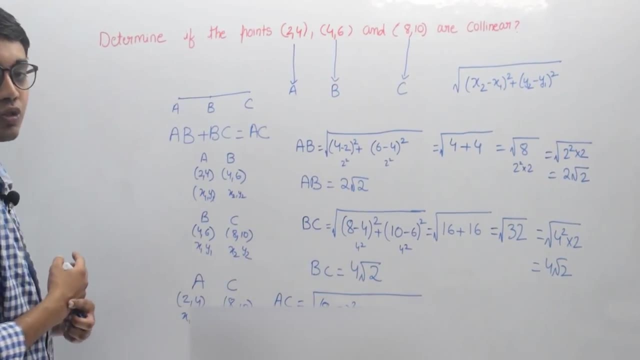 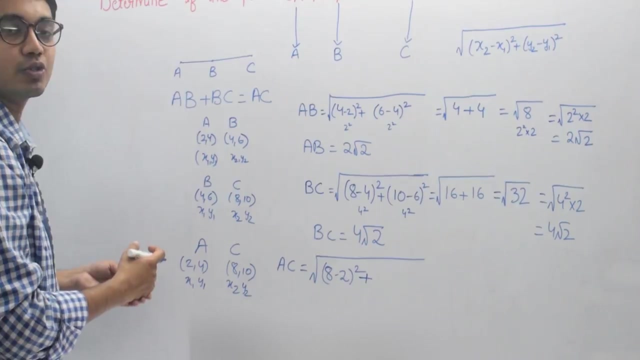 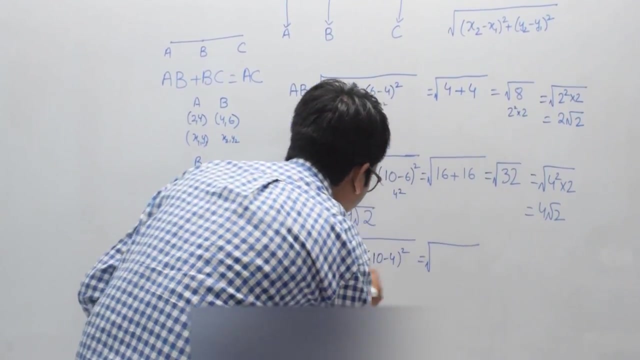 square root of 8 minus 2 whole square, that is, x2 minus x1 whole square. So AC will be square root of 8 minus 2 whole square, that is x2 minus x1 whole square. So this will be square root of 8 minus 2 is 6 and 6 square. we will have here 10 minus 4 is 6 and we